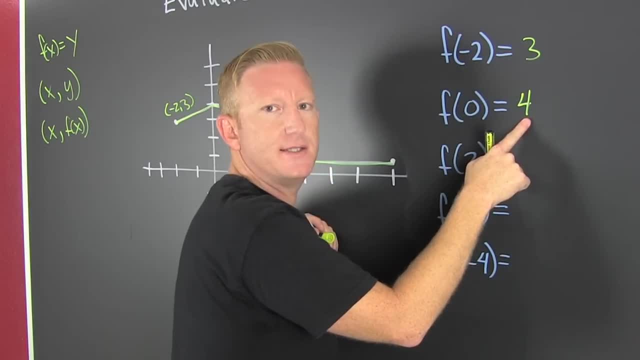 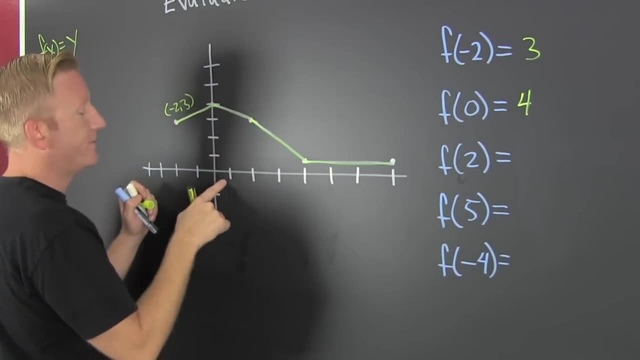 Is 4.. It's asking: what is the y value when x is 0?? Now it's asking what is the y value when f is 2? Or f of 2.. So we do go over to f is 2 and we see that that's going to be. 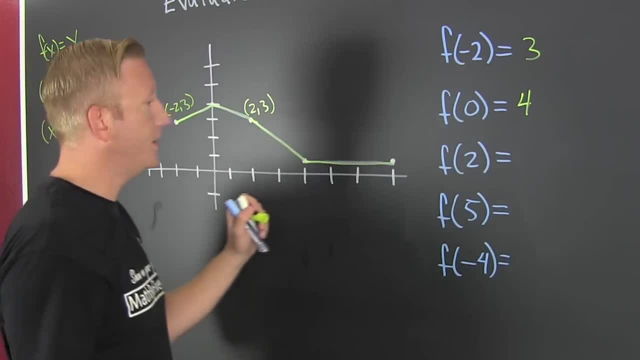 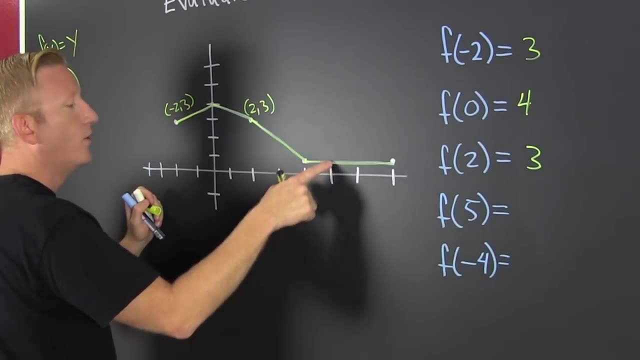 3.. That's 2 comma 3.. Oh boy, So that's 3.. More 5.. X is 5.. That's right there. What's y? Y is 1.. That's 5, 1.. All right. 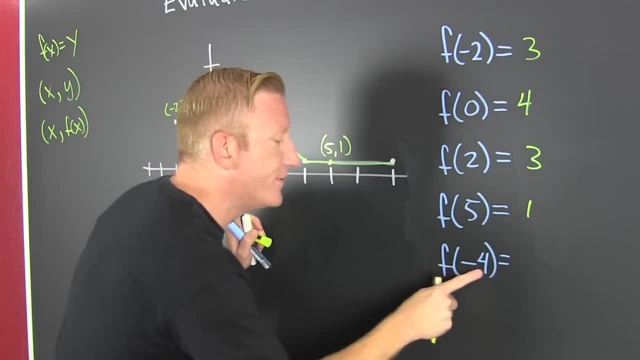 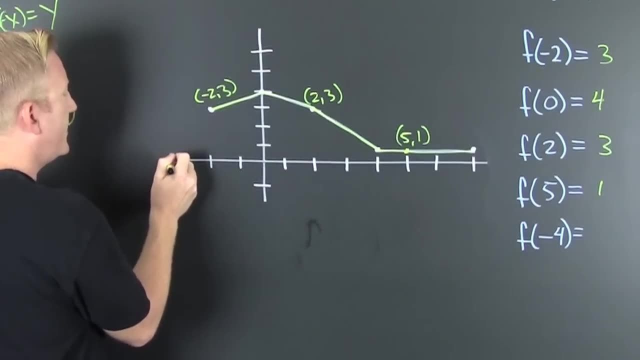 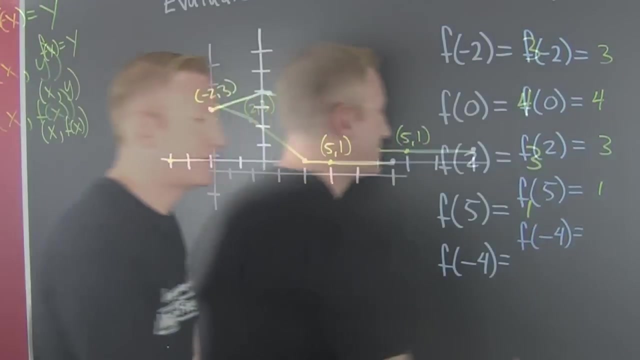 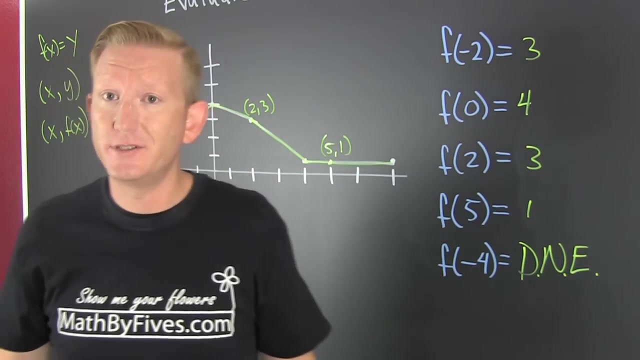 So that's 1. One more F of minus 4.. I want to explore what happens when we go over here to minus 4.. Now you're sitting here and you look high and you look low and you don't find anything. This does not exist, And that's pretty much how you evaluate a function from. 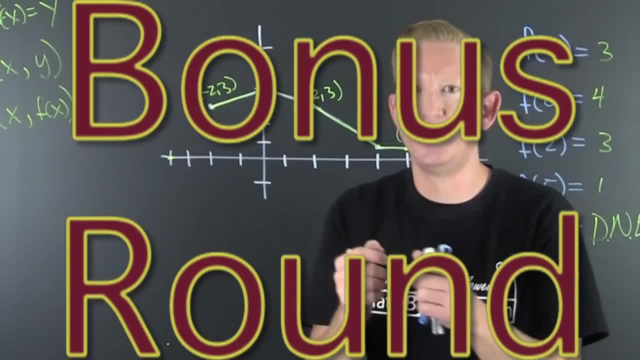 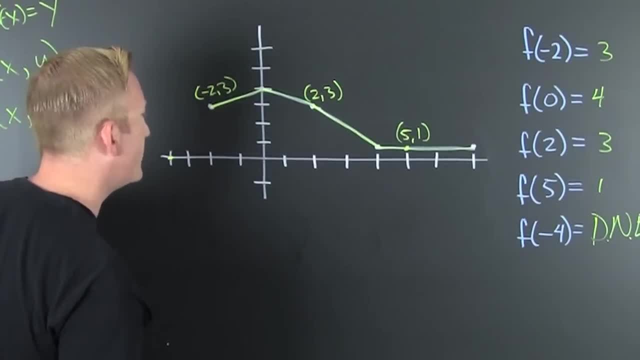 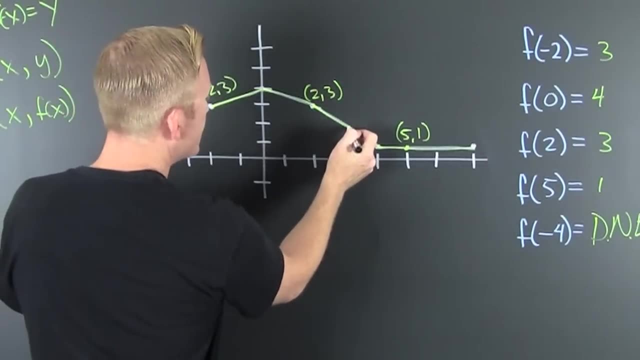 a graph Bonus round. Oh boy, Oh sure, What's this bonus round? This bonus round is when I found boom, wait, wait, wait. Oh, I'm kind of looking at this point right here. Yeah, that point, right, there is going. 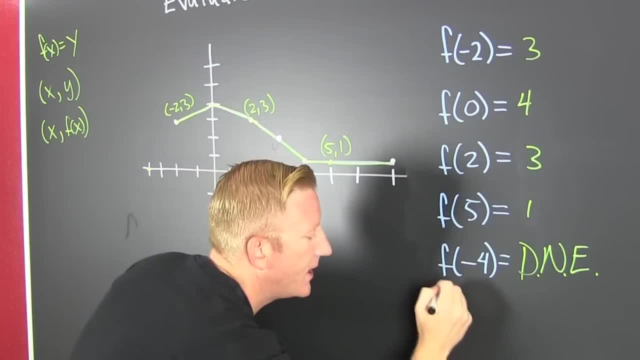 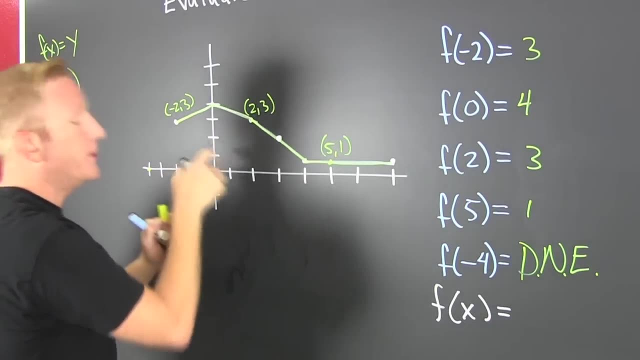 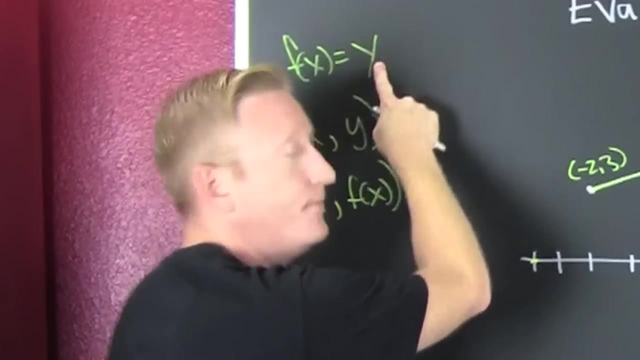 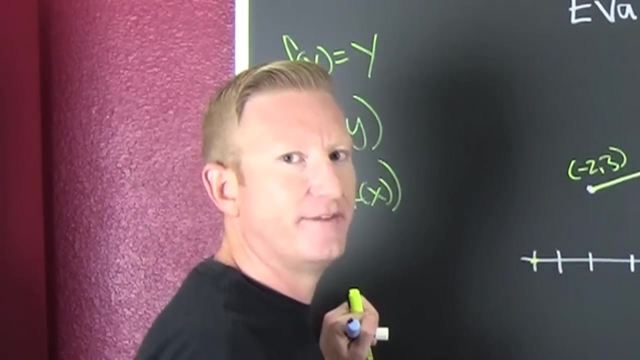 to be fine. That point right, there is going to be fine. This time I want to find the x value when y is equal to 2. When y is equal to 2.. Look, This time we gave a y and we're trying to find the x. I know why. I have a couple. 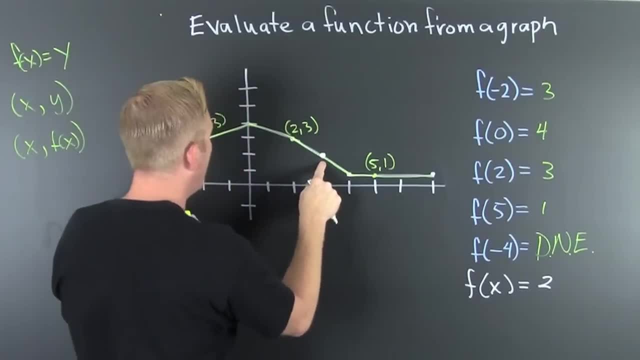 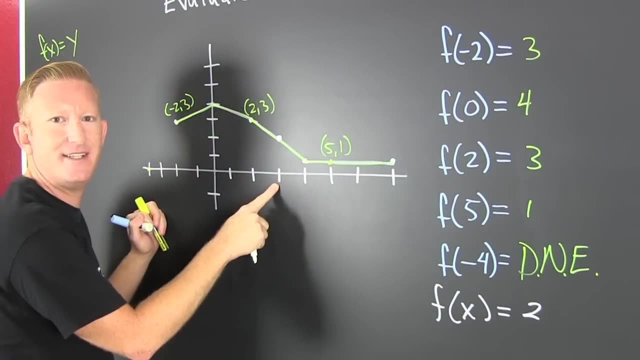 of x's. Anyways, okay, So then I'm over here, Boom, Uh-huh, My y is 2.. What do I want to find? My x? Actually, no, I don't, But if I were she's acting like she was 2.. 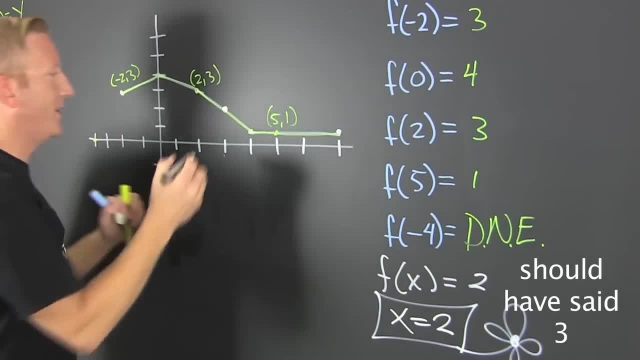 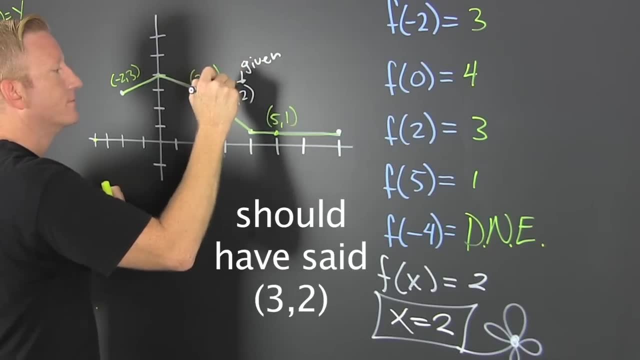 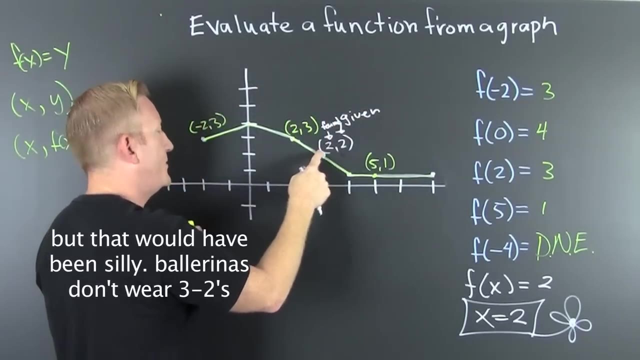 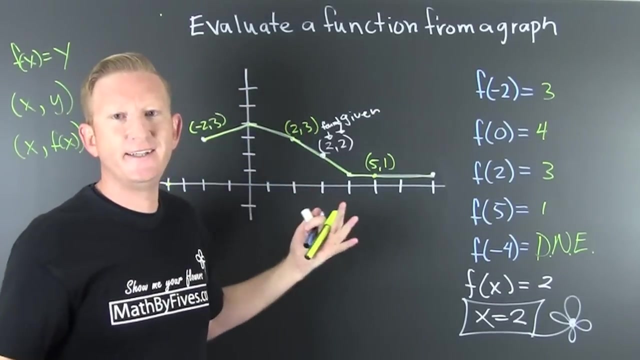 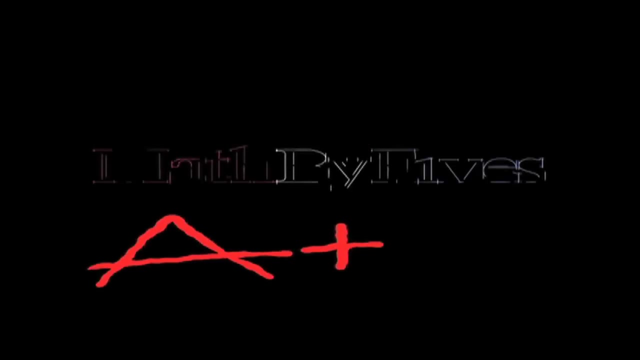 Because what does a ballerina wear? They gave us 2.. We found 2.. Clean. We're sorry, The number you have dialed is not in service at this time. Okay, All right. So what's going to be 2??